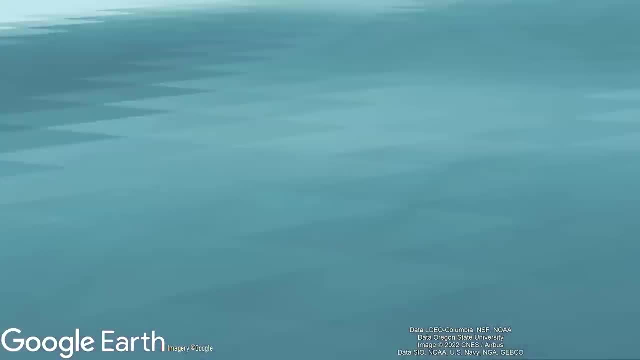 north of the island of Ta'u. At that very location are a series of two. north of the island of Ta'u. At that very location are a series of two. north of the island of Ta'u, At that very location are a series of two northward trending ridges which likely represent a chain of underwater volcanic cones. 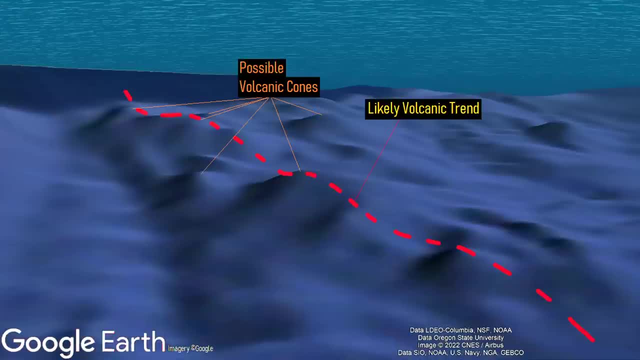 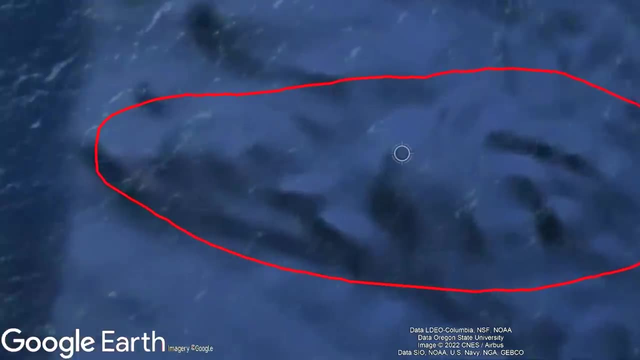 Not much is known about this area, but it would not be all that too surprising if one or more of these vents had erupted at some point in the last 10,000 years. We simply do not know yet, as the water depth in the area is between 700 meters and 2700 meters. 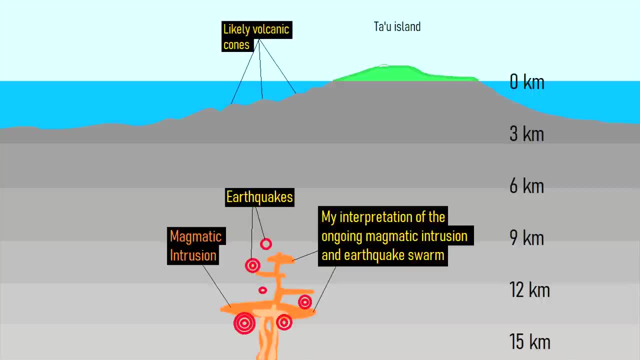 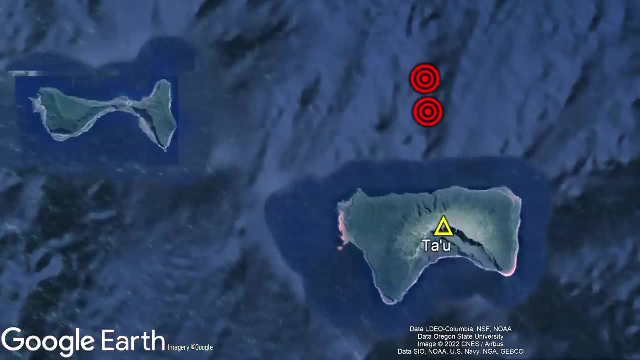 This means that, at the very shallowest, magma is still slightly more than 7 kilometers below the ocean bottom, And, since the epicenter of the earthquakes had been narrowed down, its location has not further moved. In other words, it is quite likely that, whatever 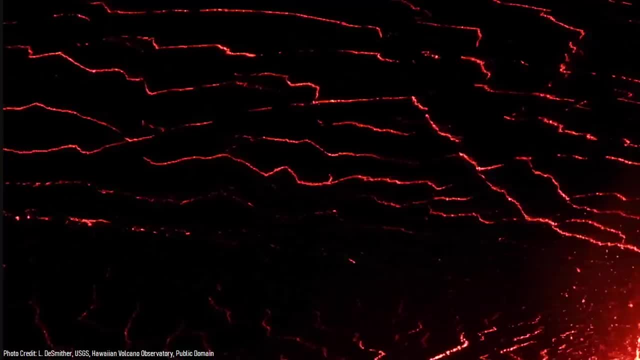 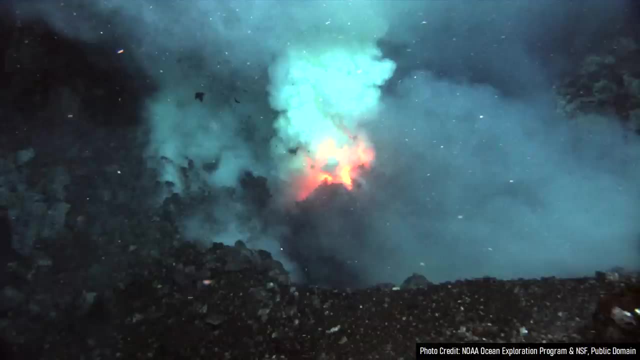 magmatic intrusion caused. all of this unrest has likely stalled and is not advancing further towards the crust. Thus, while a new volcanic eruption could still occur at a vent to the north of the island, the odds of this are not necessarily high. These odds have further declined as beginning. 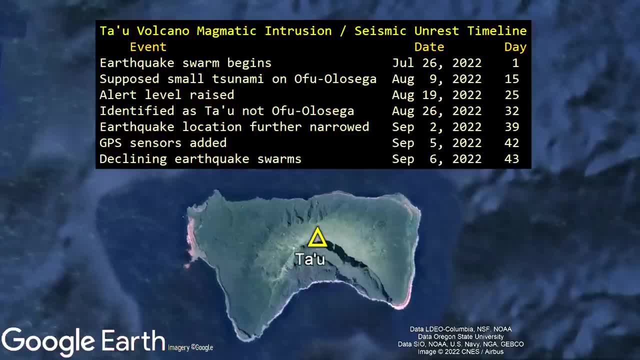 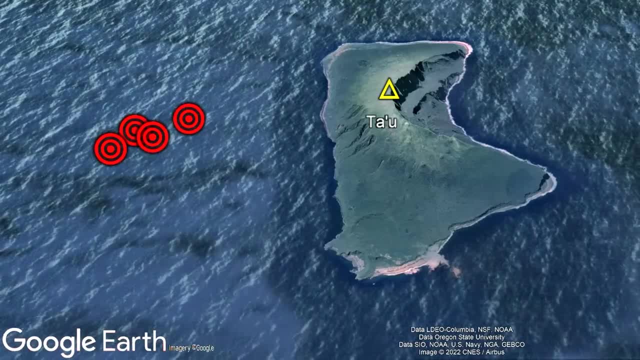 on September 6th, the frequency and rate of larger magnitude earthquakes has decreased. Although, as of the making of this video, the number of earthquakes has stabilized slightly. In terms of the broader context, it is unclear what this intrusion might represent. 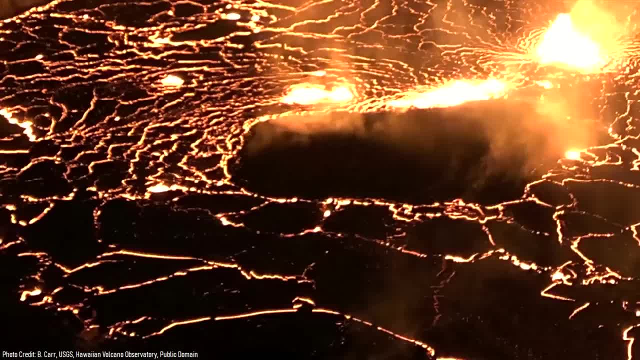 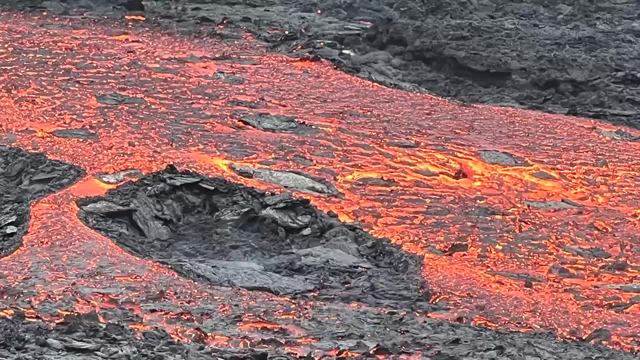 It could simply be an isolated event, Or it might signal the first of several magmatic intrusions, some of which might be more likely to cause a submarine eruption or non-submarine eruption on Ta'u island. After all, the area is highly volcanically active. 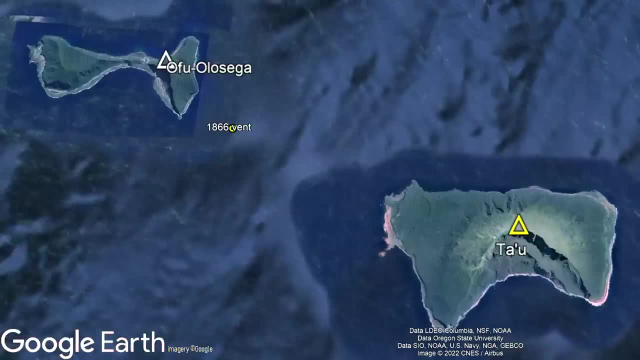 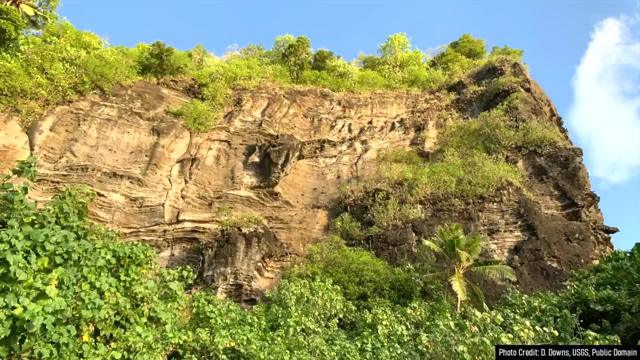 as, for example, the adjacent Ofulolosega volcano produced a submarine eruption in 1866.. However, since the exact record of eruptions at Ta'u has remained unclear and the eruptions on land appear to be primarily effusive, with some explosive eruptions near water, 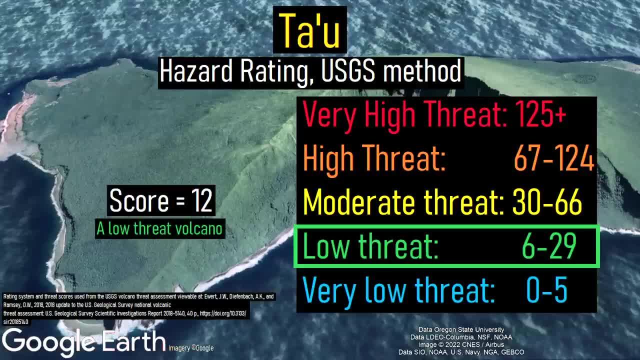 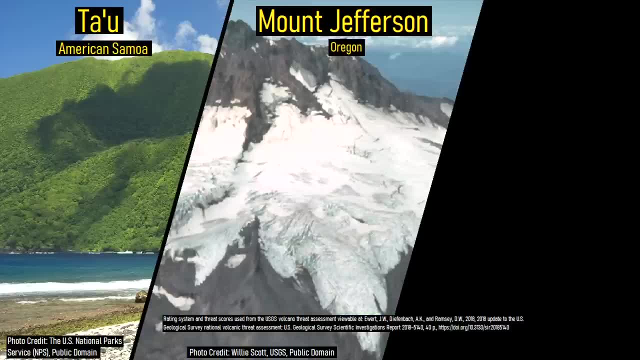 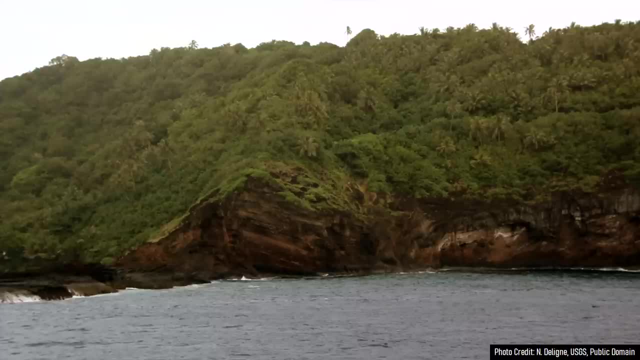 this volcano was assigned a low threat rating, just like its neighbor in the US Geological Survey volcano threat assessment. Two other volcanoes which have approximately the same threat score are Mount Jefferson in Oregon and Craters of the Moon in Idaho. What I am trying to say is that it is quite interesting. the volcano